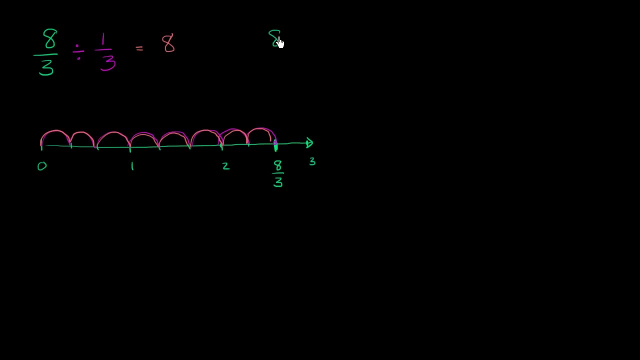 So another way of thinking about it is that 8 thirds divided by 1 third is the same thing as 8 thirds divided by 1 third, 8 thirds times 3.. And we could either write it like this, We could write times 3 like that: 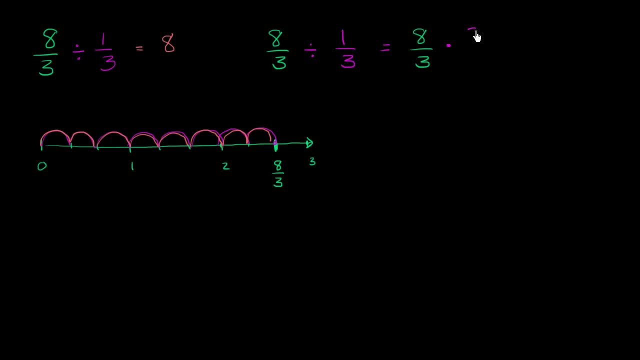 Or if we want to write 3 as a fraction, we know that 3 is the same thing as 3 over 1.. And when we already know how to multiply fractions, multiply the numerators 8 times 3.. So you have 8.. 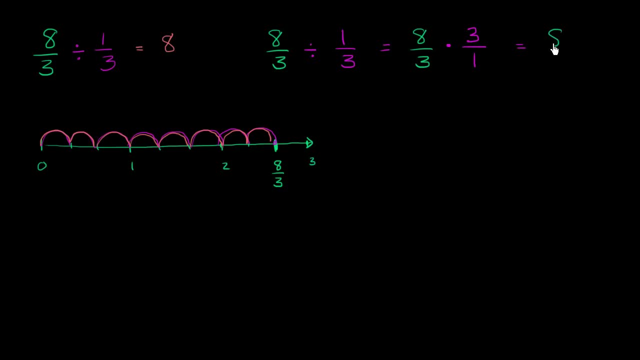 Let me do that same color. You have 8 times 3 in the numerator, now 8 times 3.. And then you have 3 times 1 in the denominator, which would give you 24 thirds, which is the same thing as 24 divided by 3, which, once again, 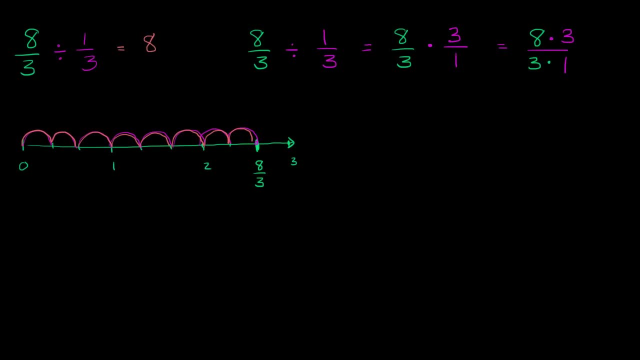 is equal to 8.. Now let's see if this still makes sense, Instead of dividing by 1 third, if we were to divide by 2 thirds. So let's think about what 8 is. Let's think about what 8 is. 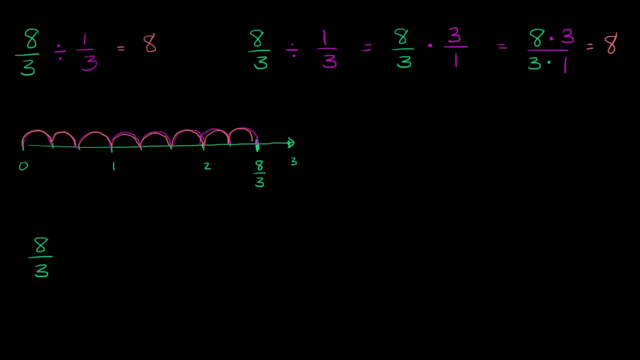 Let's think about what 8 is. Let's think about what 8 thirds divided by 2 thirds is Divided by 2 thirds. Well, once again, this is like asking the question if we wanted to break up this section from 0 to 8 thirds. 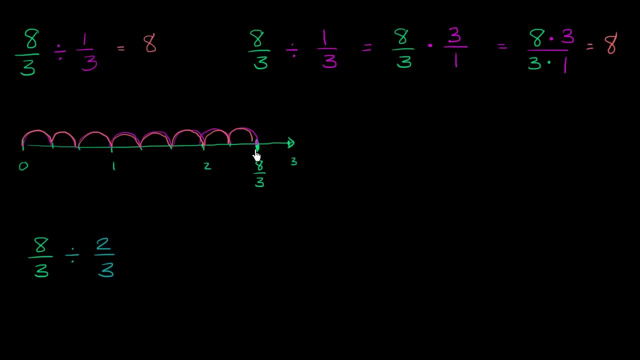 into sections of 2 thirds or jumps of 2 thirds. how many sections or how many jumps would I have to make? Well, let's think about it. One jump, but it's in a different color. We could make one jump and that's. 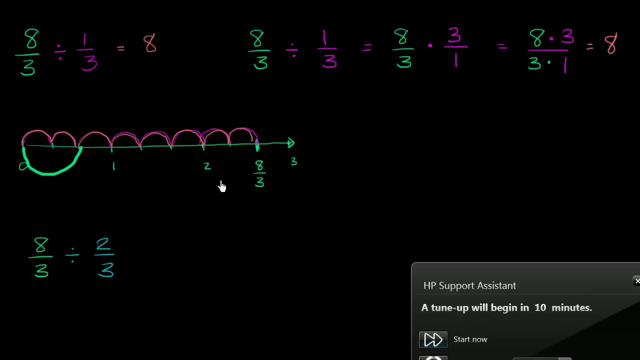 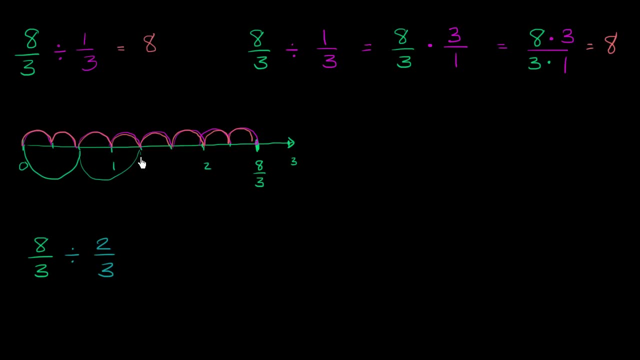 the same color as my 8 thirds, We could do one jump. My computer is doing something strange. We could do one jump, two jumps, three jumps and four jumps. So we see 8 thirds divided by 2 thirds is equal to 4.. 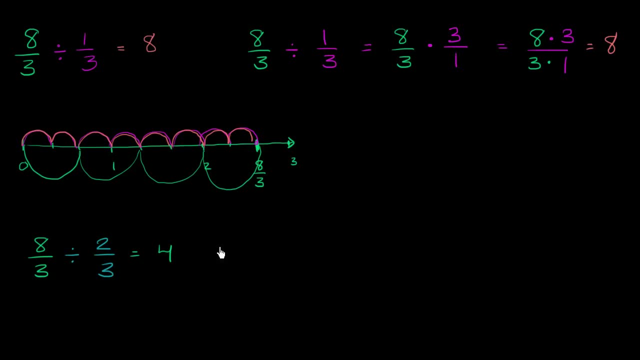 Now, does this make sense in this world right over here? Well, if we take 8 thirds and we do the same thing, saying: hey look, dividing by a fraction is the same thing as multiplying by a reciprocal. well, let's multiply by 3 halves. 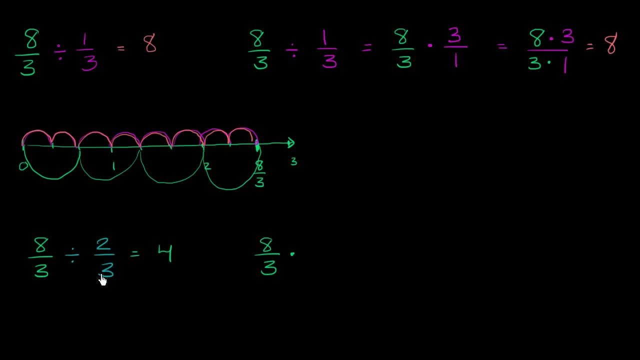 Let's multiply by the reciprocal of 2 thirds. So we swap the numerator and the denominator. So we multiply it times 3 halves. And then what do we get In the numerator? once again, we get 8 times 3, which is 24.. 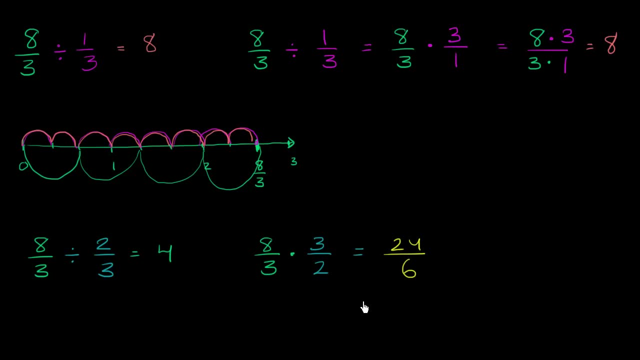 And in the denominator we get 3 times 2, which is 6.. So now we get: 24 divided by 6 is equal to 4.. Now does it make sense that we could do this? Well, we got half the answer. 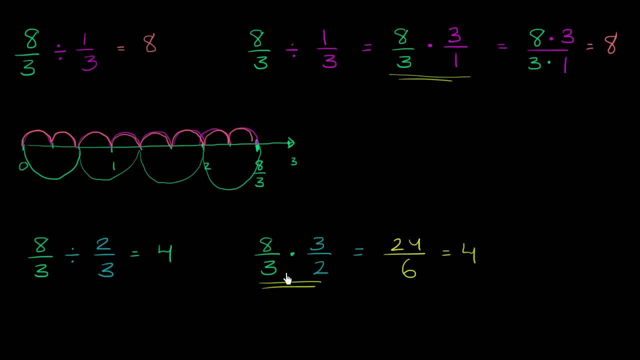 If you think about the difference between what we did here and what we did here, these are almost the same, except here we really just didn't divide. or you could say: you divided by 1, while here you divided by 2.. Well, does that make sense? 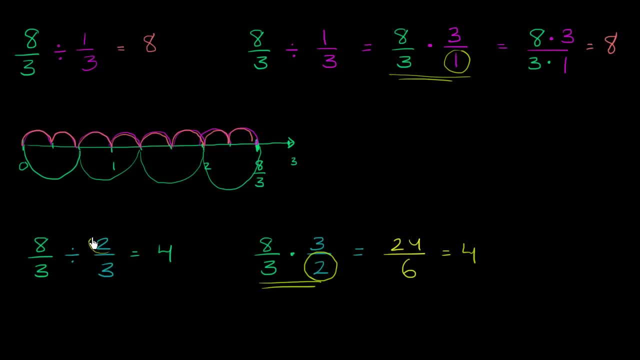 Well, sure, because here you jumped twice as far. You jumped twice as far so you had to take half the number of steps. And so in the first example you saw why it makes sense to multiply by 3. When you divide by a fraction for every whole, 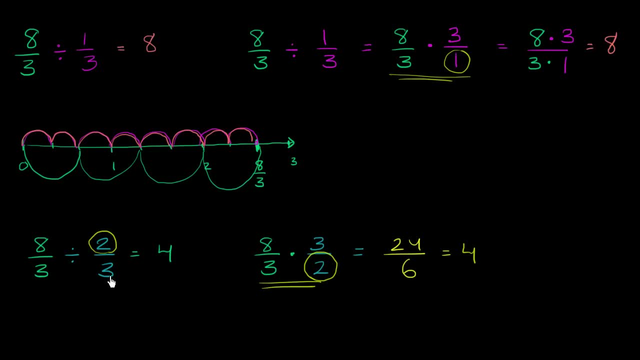 you're making 3 jumps. So that's why, when you divide by this fraction, you multiply. or when you divide whatever's in the denominator, you multiply by it. And now, when the numerator is greater than 1, every jump, you're going twice as far. 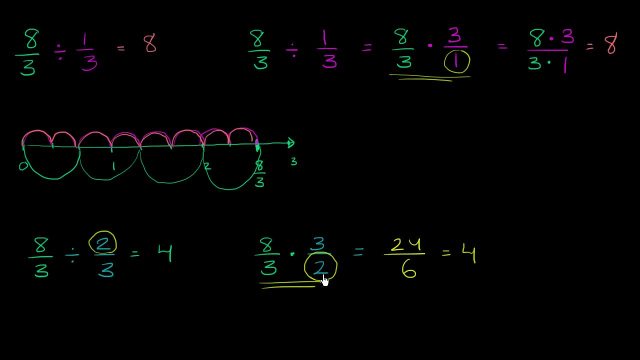 as you did in this first one right over here, And so you would have to do half as many jumps. Hopefully that makes sense. It's easy to think about just mechanically how to divide fractions, Taking 8 thirds divided by 1 third. 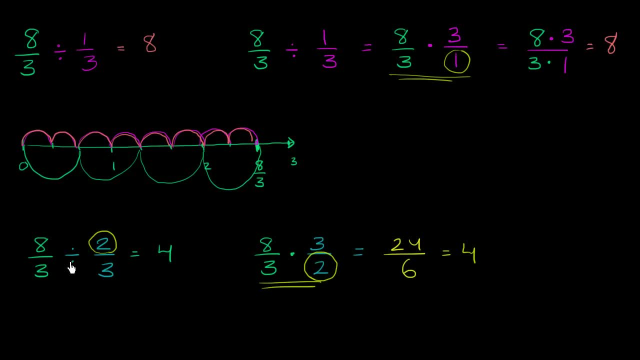 is the same thing as 8 thirds. So 8 times 3 over 1, or 8 thirds divided by 2 thirds is the same thing as 8 thirds times 3 over 2.. But hopefully this video gives you a little bit more of an intuition. of why this is the case. 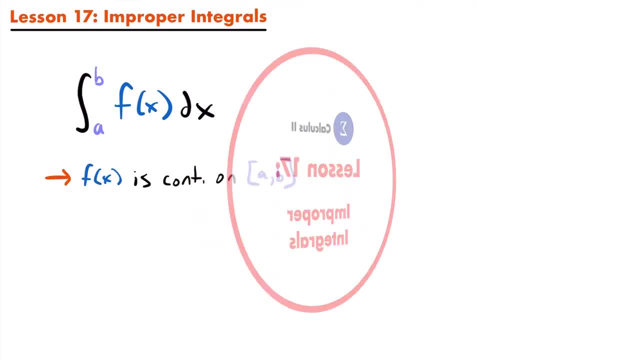 Welcome back. In this video you will learn how to solve improper integrals. Let's get to it Alright. so so far in calculus, when we have been evaluating definite integrals, we have been integrating functions over a range of values for which that function is continuous right. So when